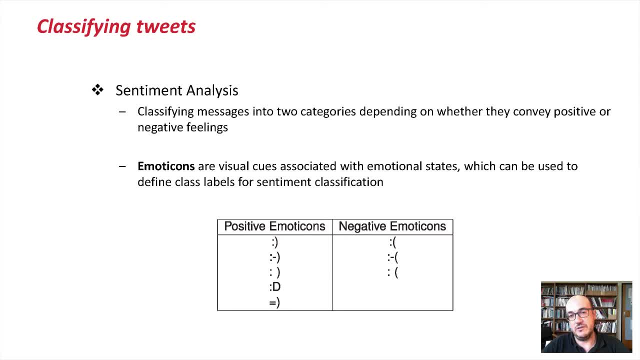 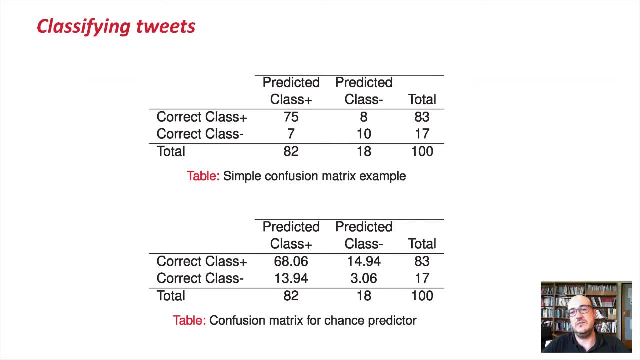 what is the current polarity, what is the current sentiment around any specific tweet? So we can actually use this information to classify tweets if we want a specific product or company or topic. An important thing that we need to look at when we are classifying tweets is that if 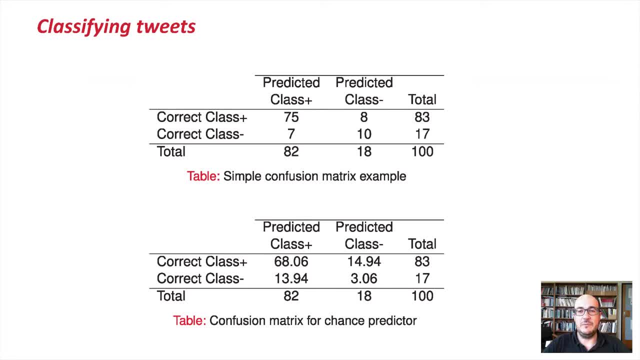 data is balanced or not. So let's look at an example. so in this simple confusion matrix, what we see is that we are predicting 82% as positive and 18% of the instances as negative. What we see is that we are classifying correctly the positive class, 75% of the instances as positive, and 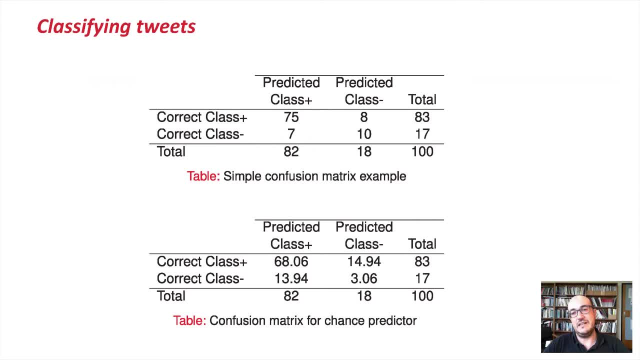 then we're classifying the negative class- 75% of the instances- as positive- and that's the most important thing- and we are correcting the negative class 10% of the instances. So our accuracy in this case is 85%. Is this a good performance? 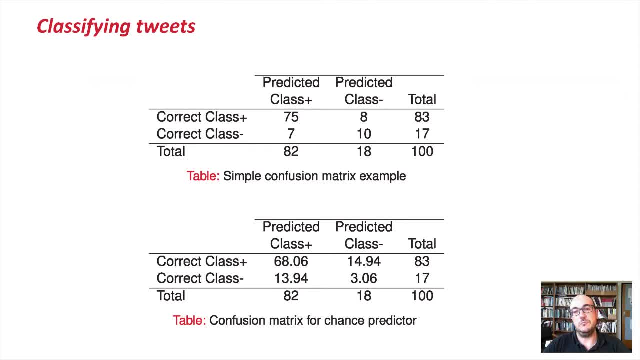 To answer this one way is that we can look at a random classifier. Imagine a random classifier that is predicting randomly but is following the same distribution between positive class and negative class. So this is the confusion matrix in the bottom. So there we can see that this classifier is getting also 82% of the instances as positives. 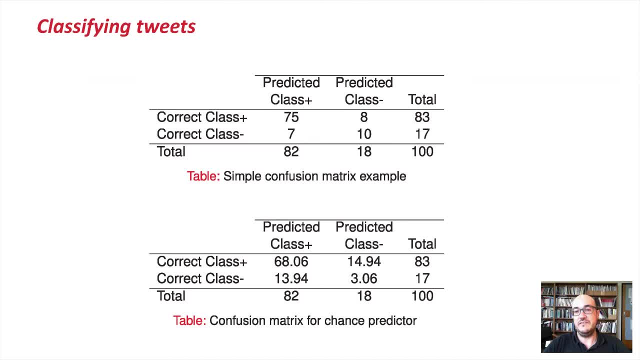 and is predicting as negative 18%. Interesting thing is that it's predicting the positive class correctly 68% of the time and the negative is predicted correctly 3% of the instances. So that means that the accuracy here is 71%. So that means that if our classifier is predicting 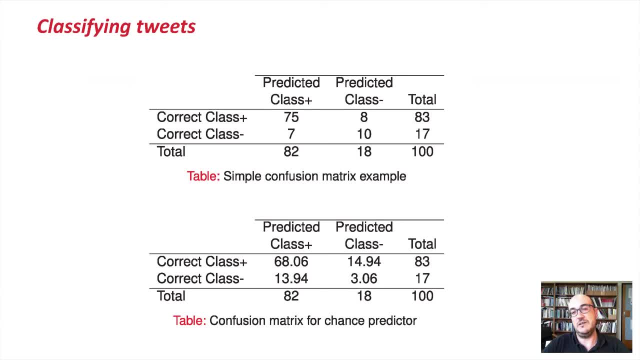 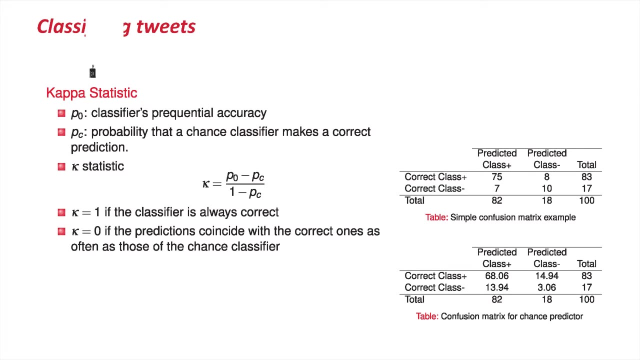 with accuracy higher than this, then we can say that it's a good classifier, But if it's predicting less than this 71%, then our classifier is not doing quite well To see this. this is, as you may know, there is this Kappa statistic measure- that what it's measuring is this difference. 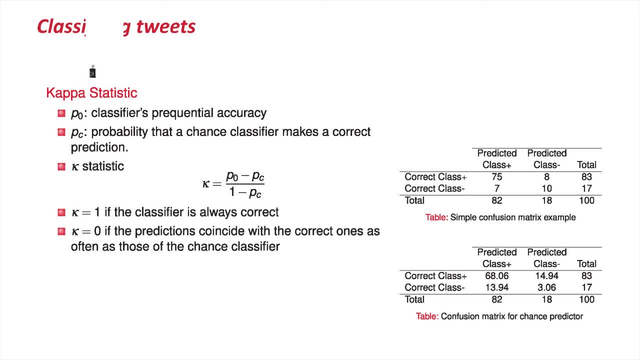 The difference between the accuracy of our classifier with the accuracy of a random classifier that is predicting using the same distribution of classes. So basically, Kappa statistics computes this difference and then it adds a normalizing factor, so we get a value of Kappa between 0 and 1.. 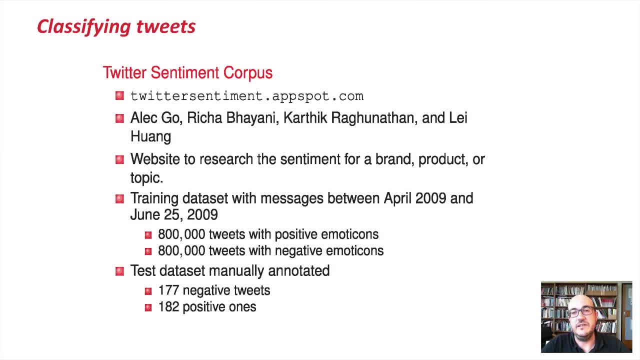 Now let's look at an application. So there is this Twitter sentiment corpus that was made by students at Stanford that contains tweets recollected between April 2009 and June 2009, where there are 800,000 tweets with positive emoticons and 800,000 tweets with negative emoticons. 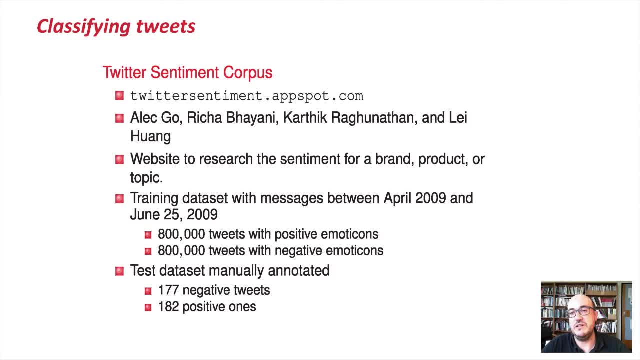 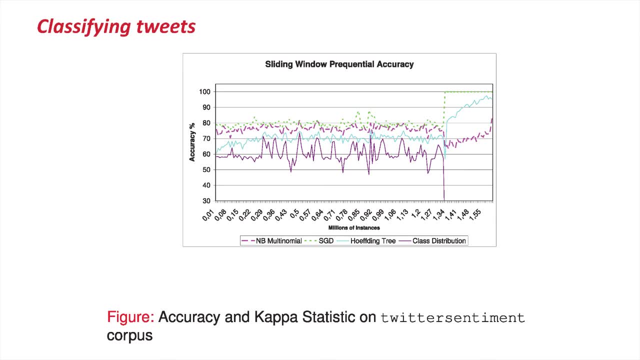 If we do a frequency evaluation using these tweets and we use a naive Bayes multinomial classifier, stochastic gradient descent classifier and a Hoeffding tree, what we see is that at the end of the stream, the stochastic gradient descent classifier gets an accuracy of 100%. 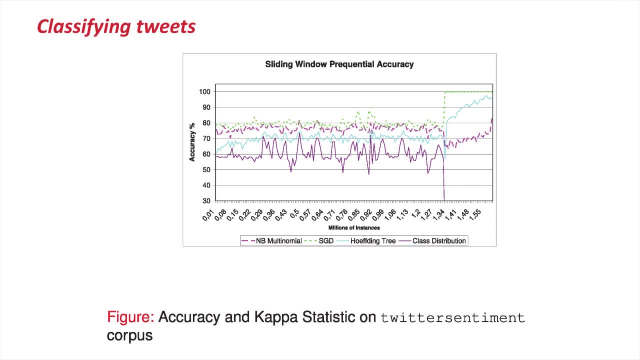 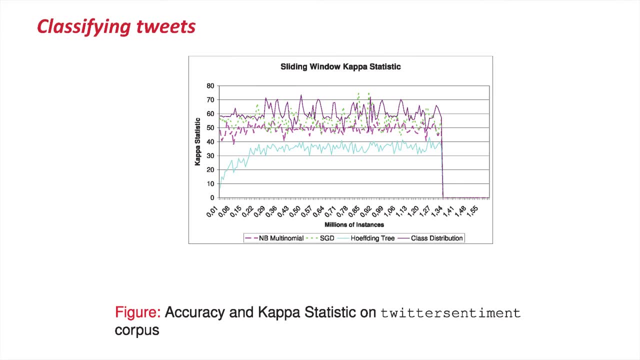 So this is something that is not normal, And then it's nice to see why it's happening this. If we look at the Kappa statistic, what we see is that, at the moment that the accuracy goes up to 100%, the Kappa statistic goes down. 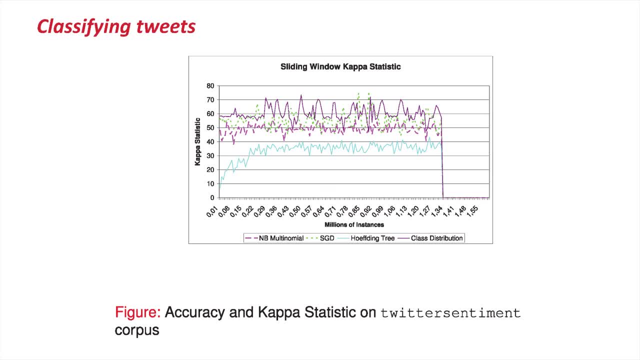 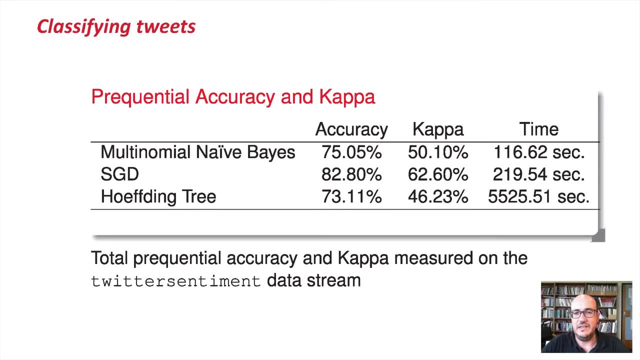 So that means that in that case the data at that point starts to be completely unbalanced and completely only belonging to one class In this data stream. if we compare accuracy and Kappa of a multinomial naive Bayes stochastic gradient descent classifier. 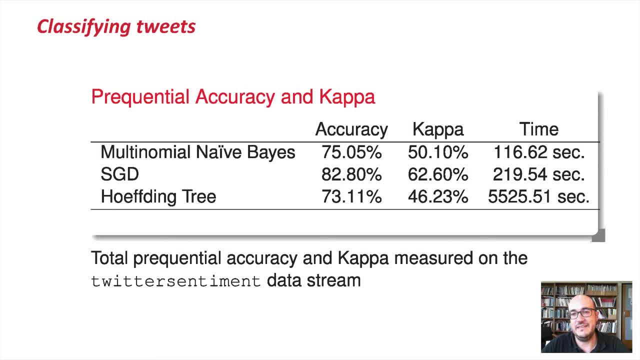 what we can see is that stochastic gradient descent is better, but this is something that maybe not applies to other data streams. What is very interesting is that in data stream mining, we should always not only look at accuracy, but also looking at the resources, at time and memory. 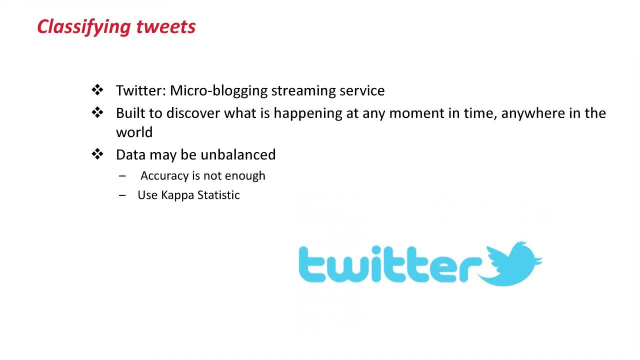 So we have arrived to the end of this lesson. So in this lesson we have seen an application of Twitter classification. Twitter is this microblogging stream service that is built to discover what is happening at any moment in time and more specifically, what is happening now. 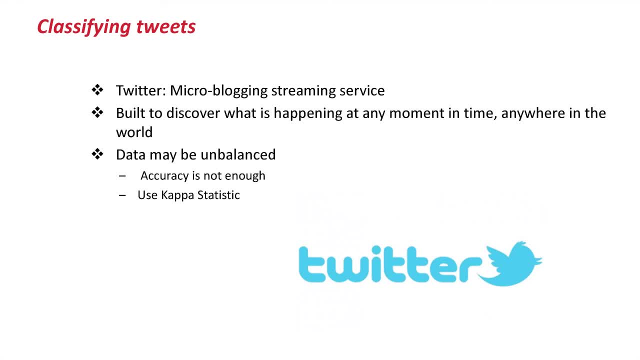 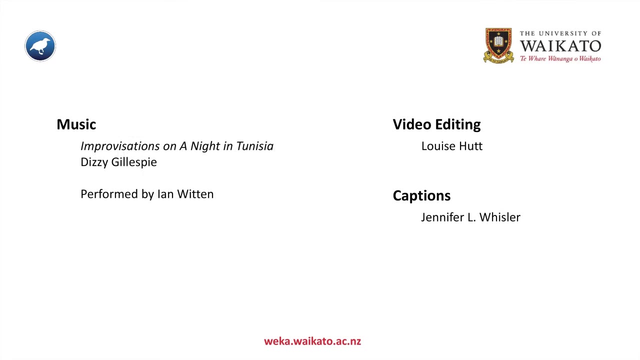 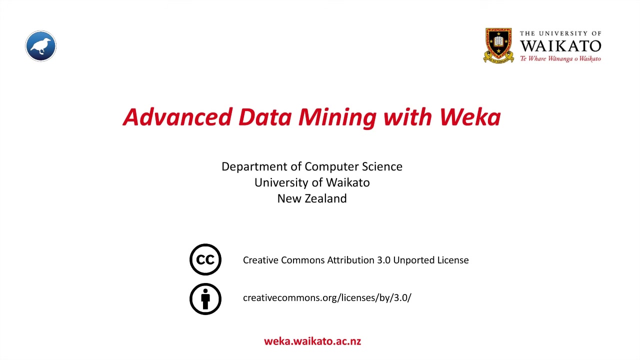 Data may be unbalanced in many data streams, so it's always important not only to look at accuracy, but also look at other measures, as Kappa statistics. So thanks for being there. I hope you enjoyed it. Bye, bye. Thank you for watching.